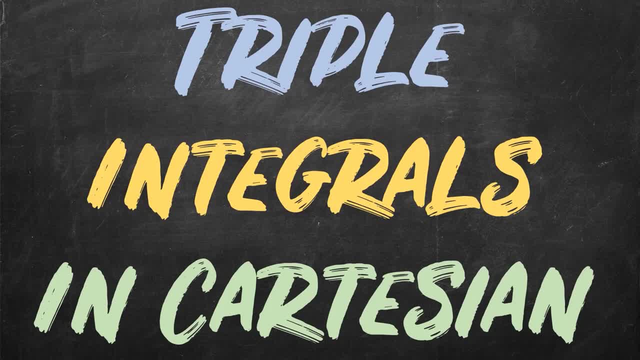 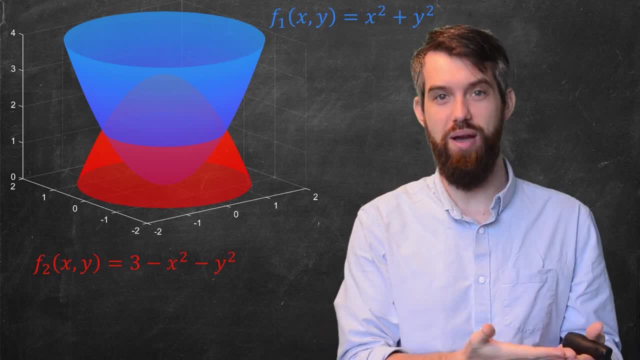 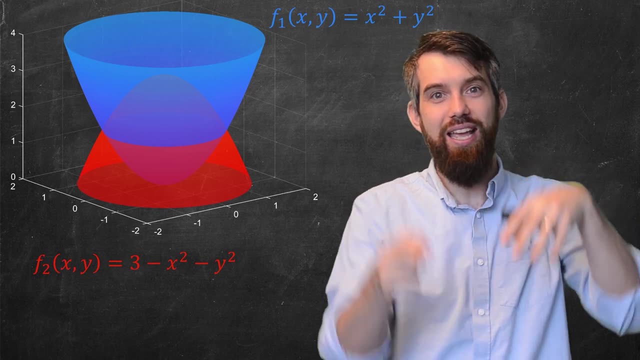 Here I have the graph of two different functions. One is the function x squared plus y squared and the other is 3 minus x squared minus y squared, And the way these functions interact is that they have an intersection and that inside of that intersection is a volume And 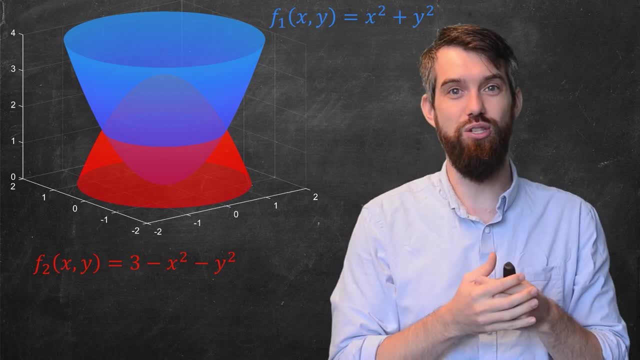 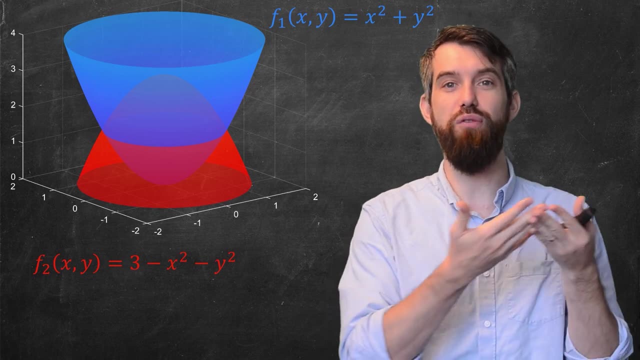 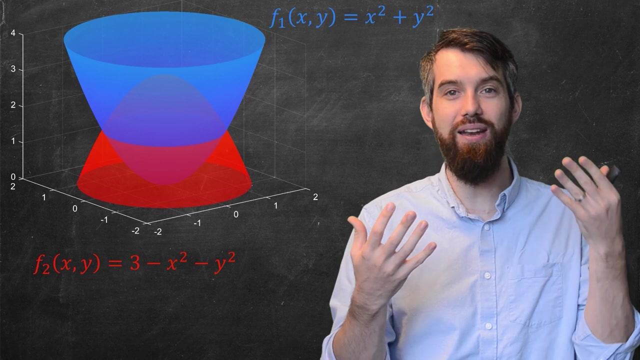 my question is: what is the volume of that region, this region in between these two different surfaces? In this video, we're going to talk about finding volumes of regions like this via triple integration, integration where I'm integrating with respect to z and y, and 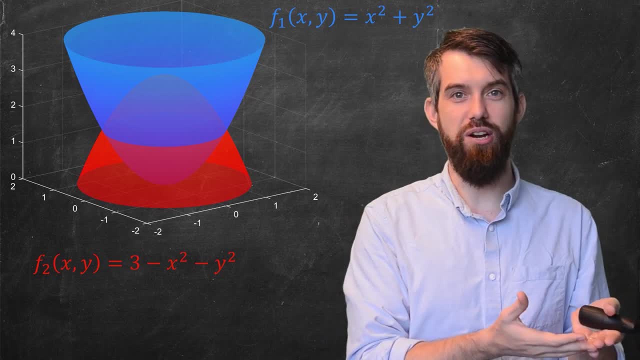 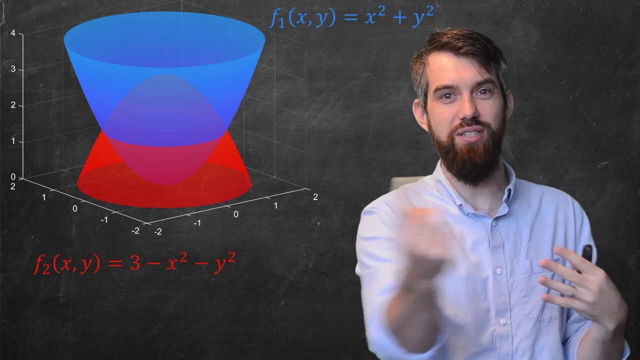 x. Now, the first thing I want to figure out here is what actually is the intersection, not just the region in between these, But if I look at this, it appears that there is a circle where these two different surfaces are going to intersect. Indeed, if I take 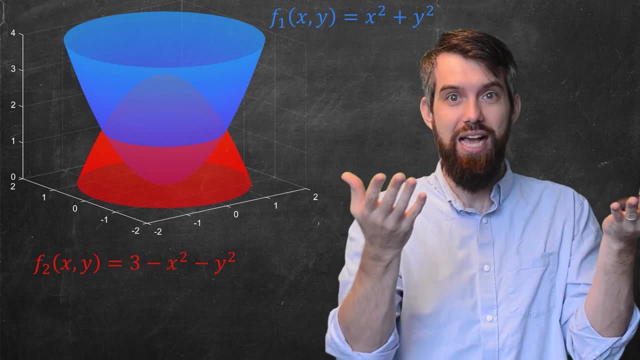 the f1 and the f2,. these are the two different surfaces, And if I take the f1 and the f2, these are the two different surfaces, And if I take the f1 and the f2, these are the z values and I set them equal to each other, then what I'm going to get is this equation: 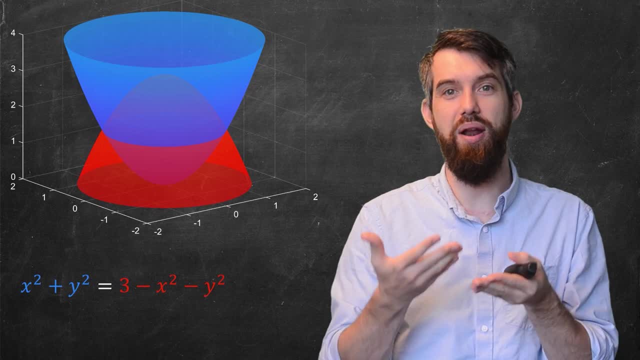 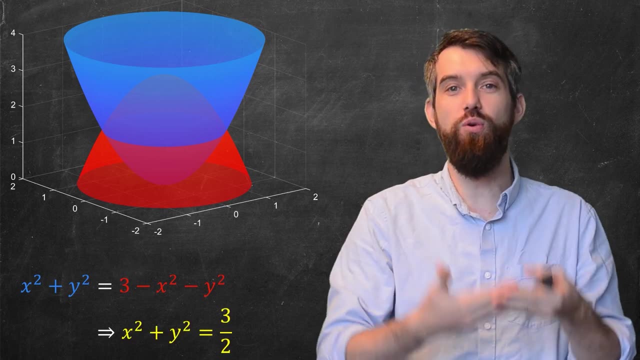 that x squared plus y squared is equal to the 3 minus x squared minus y squared. If I then add x squared plus y squared to both sides, divide out by the 2,, what I get is that x squared plus y squared is 3 halves, But x squared plus y squared equals 3 halves. 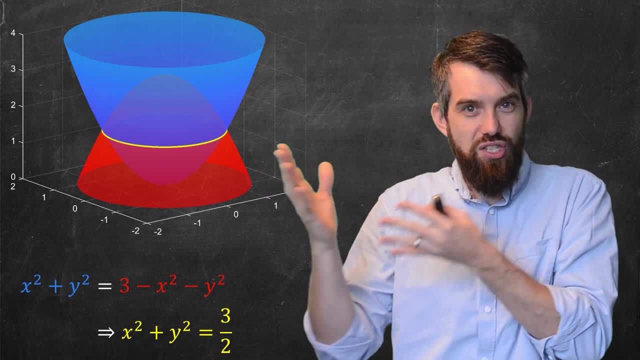 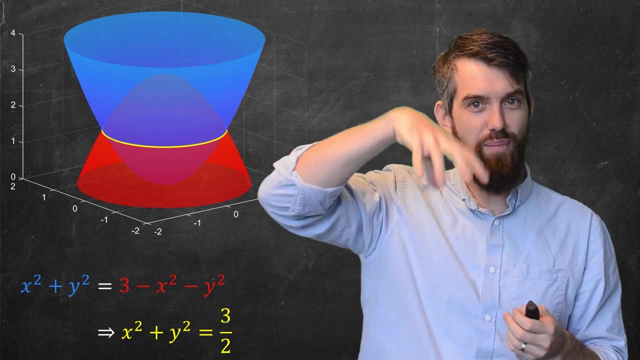 is just the equation of a circle. Indeed, on this picture, we have this circle of intersection, a circle of radius, the square root of 3 halves. I can also imagine that I'm looking straight down on this and that's going to give me in the domain just 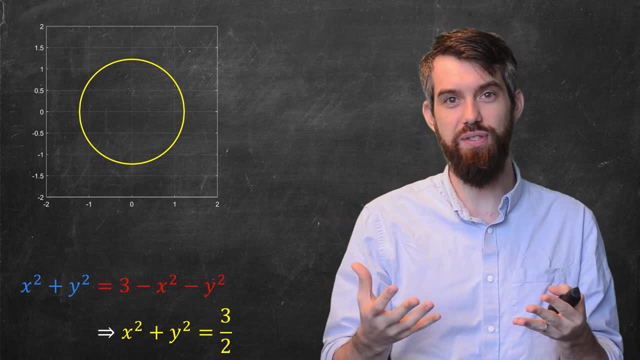 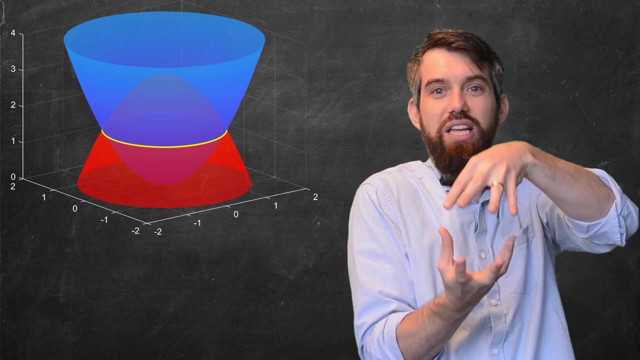 again this equation of a circle of radius, the square root of 3 halves. So when I think about this volume and trying to compute it, my first observation is that the volume is entirely constrained within this particular boundary circle, So that the x values and 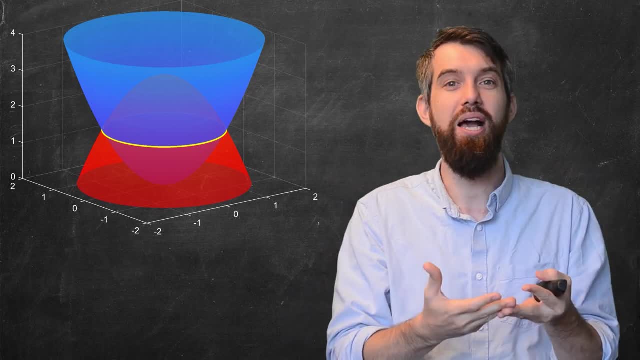 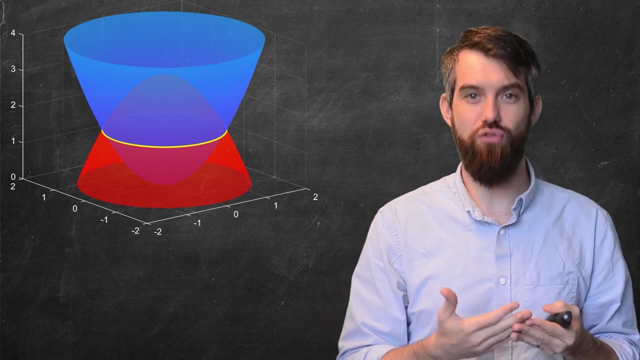 the y values when I try to figure out what those limits of integration should be. well, I'm going to get those values from this boundary circle, Okay, but what about the entire volume? Here's my strategy. I want to think of this as a triple interval. This is kind of long. 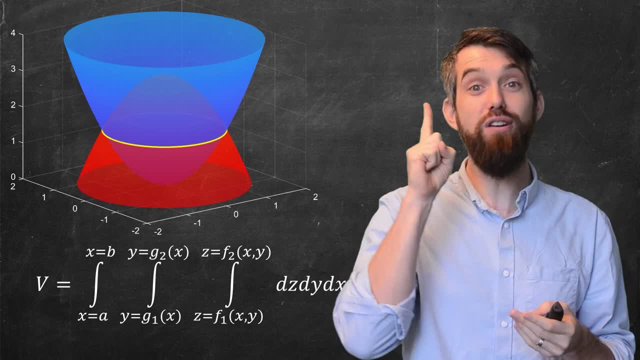 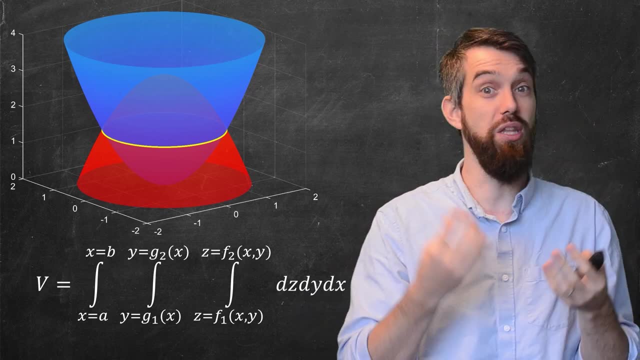 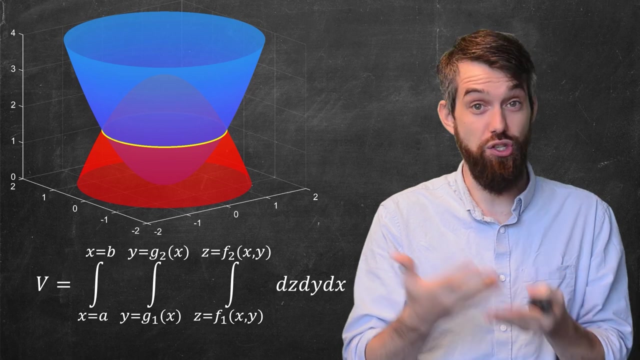 and messy. but what I have here is an interval of the function 1,, dz, dy, dx, And then my z interval has two different limits of integration: the bottom and the top function, f1 and f2.. The y interval is going to have limits of integration as well. These are functions of 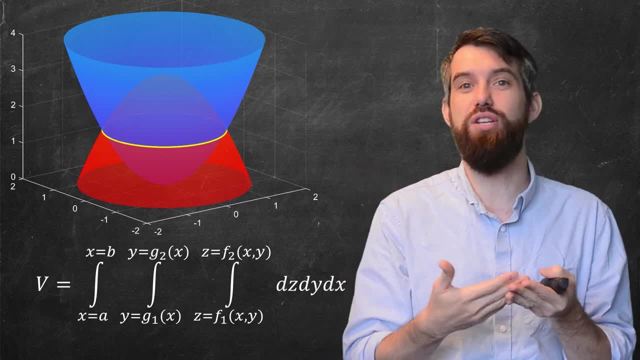 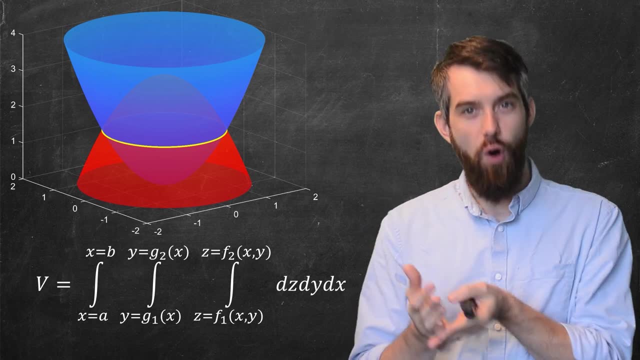 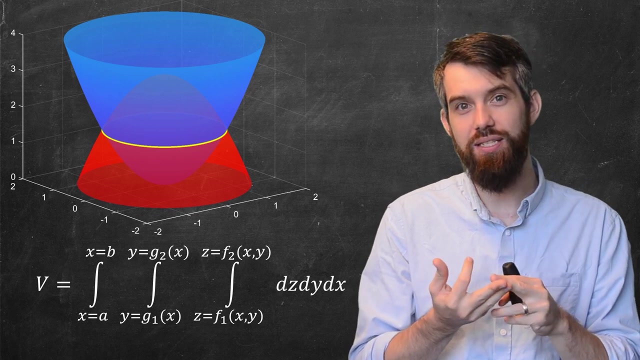 x And then the final x interval on the outside is just going to be evaluated between two different numbers. The result will be a number. The way I think of this as being a volume is that I'm adding up a lot of little volumes: dz, dy, dx. If I take this large volume and break it up into, 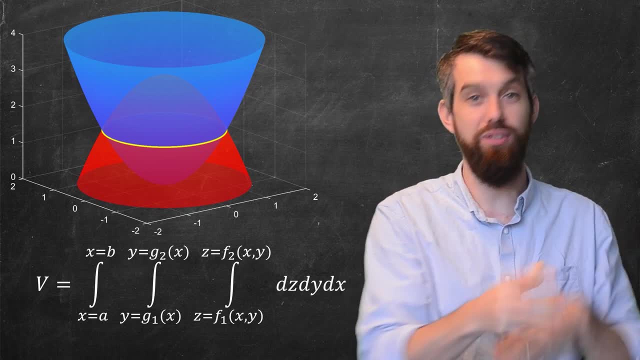 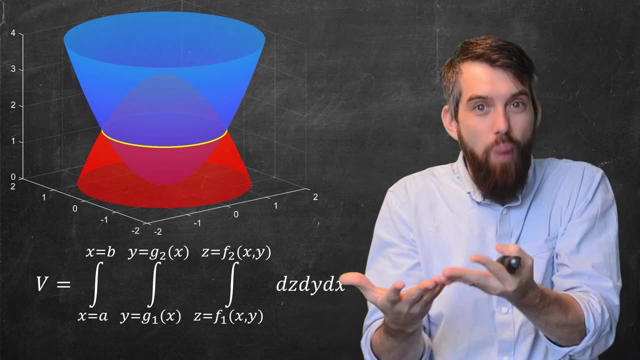 all these little individual components and I add up all of those components, I get the total volume. The interval signs are just a fancy way of saying I'm going to add up all of these small little pieces in the limit, as the m is going to infinity. So the real 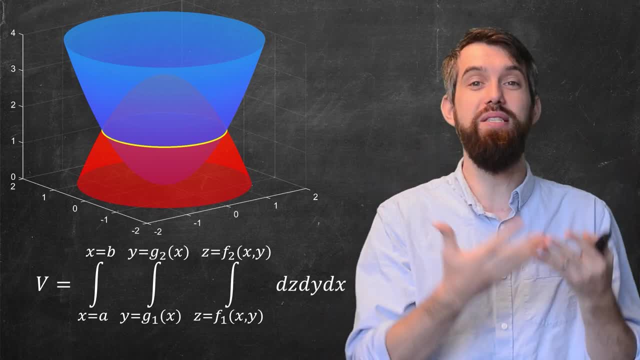 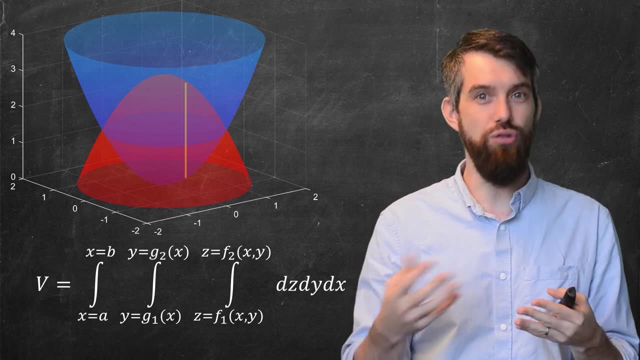 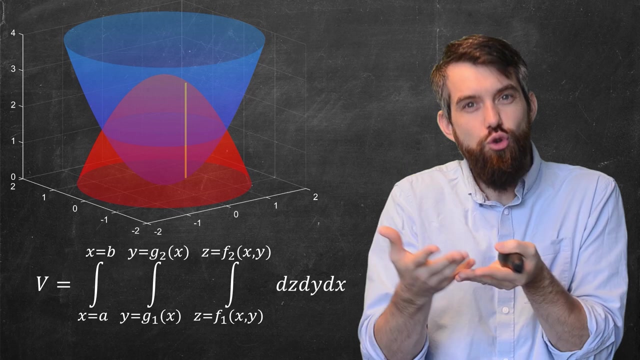 goal of this video is clear: Coming up with all of those limits of integration. If I make this a bit more transparent, what we have is that the integral with respect to z is: you choose some x value, you choose some y value, because we're going to integrate those later. So some x and y value And then 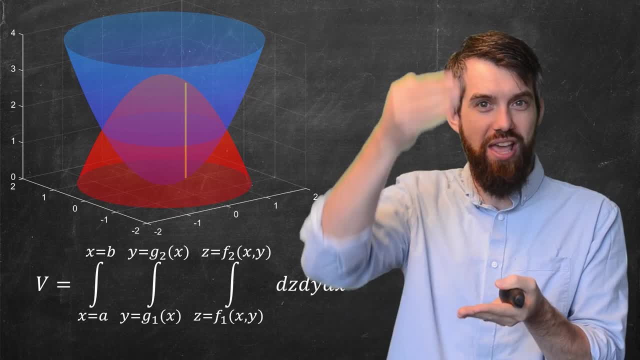 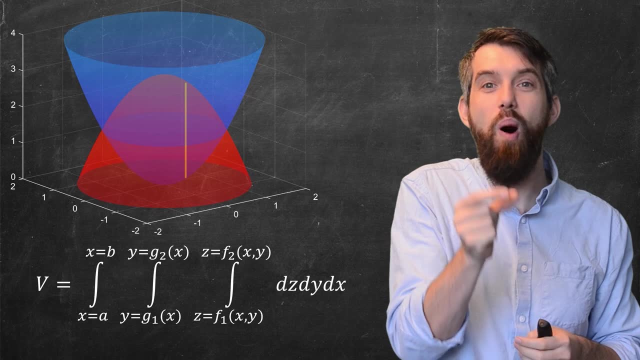 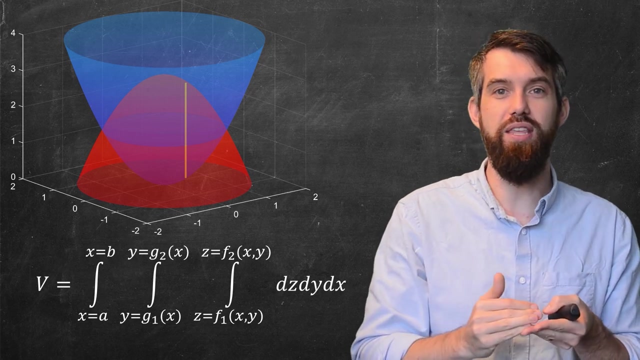 integrating with respect to z means that at that fixed x and fixed y, you have this vertical change. So I'm going to put this line, which I imagine really having a very, very small area and then some substantial finite height to it, And the bottom height of that is just the f1, and the top height of that is the f2.. So 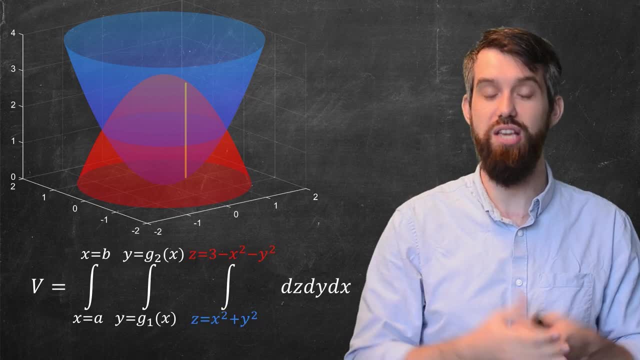 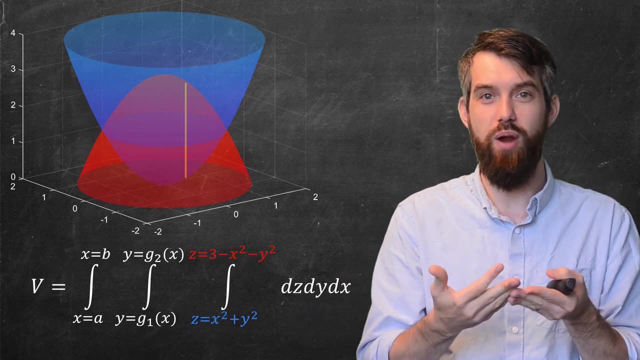 to evaluate this. all I have to do is just well substitute it. in The equations that I knew, the f1 and the f2 are going from x squared plus y squared up to the 3 minus x squared minus y squared. And that's what that little vertical strip is doing. 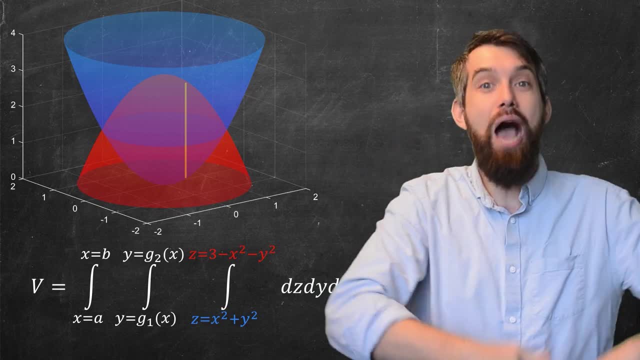 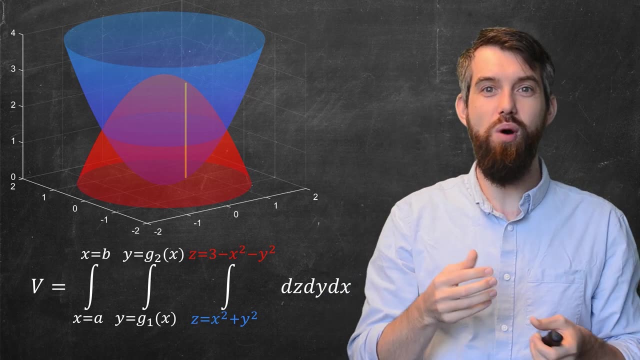 Okay, so I get that for every x and y. Now I want to integrate with respect to y. So that is this little vertical strip that I have. I want to go and send it down a lot of different y values. So then I get. 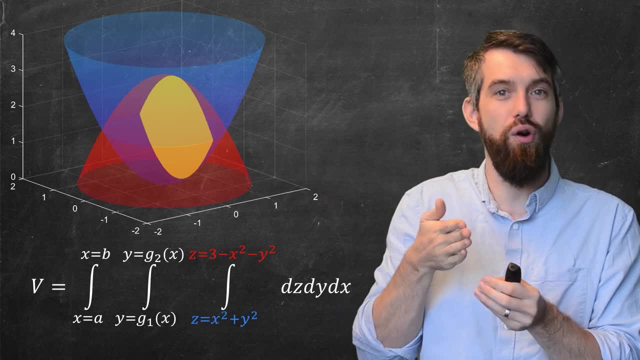 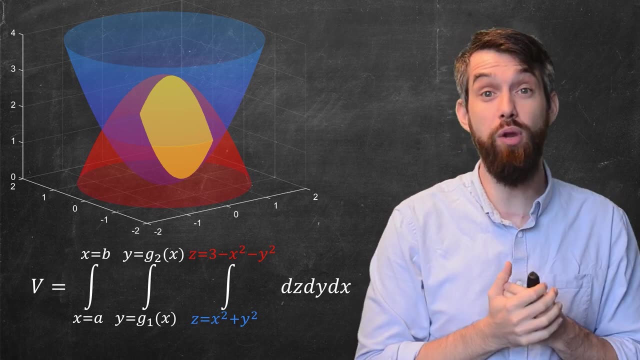 something like this: That vertical strip has moved along for all of the different y values where x is again some specified value. So I think I plugged in x equal to 0.3 when I programmed it, So I get the slice at x equal to 0.3 and as a result, 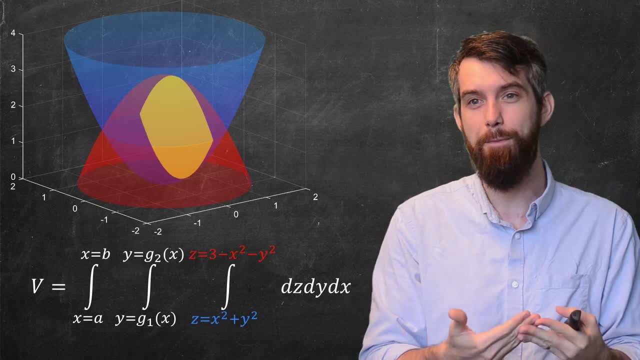 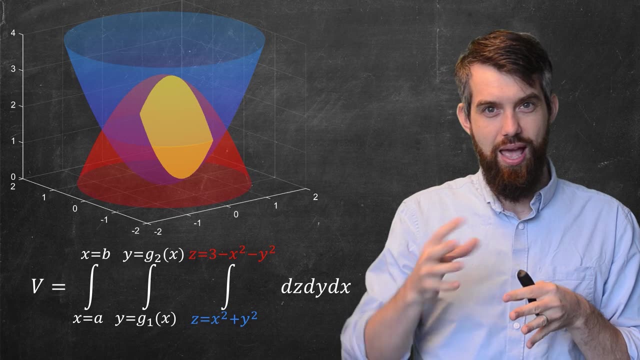 you have this little region. That's when I integrate with respect to y. Okay, but what should the limits of integration with respect to y be? If I take this picture and I look down at it from the bird's-eye view, to see just into the domain of x and y? 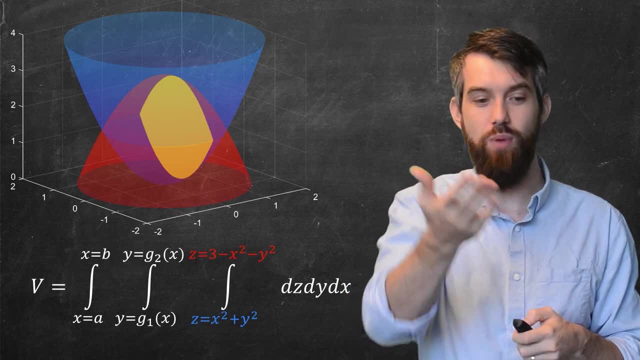 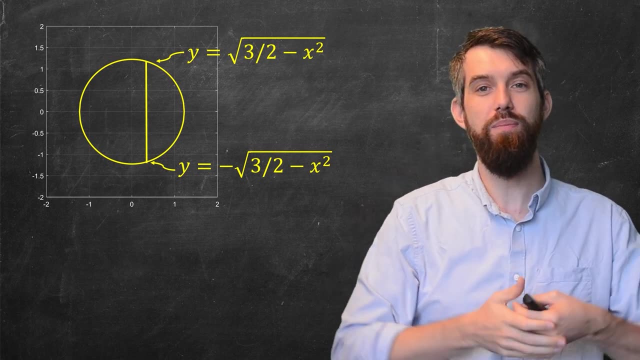 what this strip that I'm doing when I integrate with respect to y is. well, it just looks like this: I have that circle in the domain and after I integrate with respect to y, I get a vertical line, But in the domain this was an equation of a. 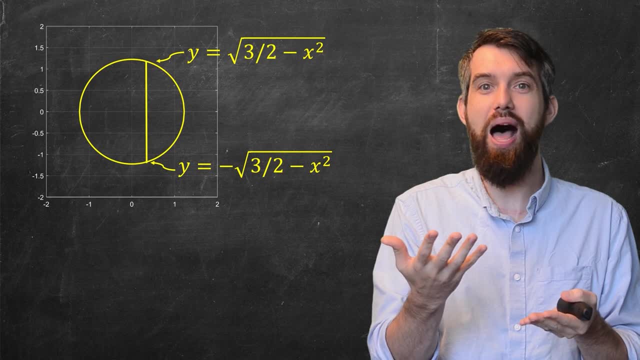 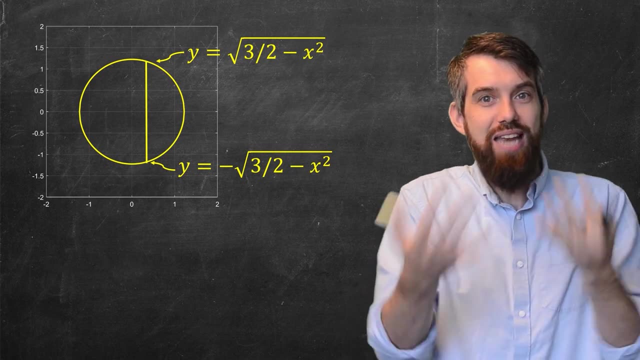 circle, So the top half of it's given by y equal to the square root of this radius of y squared, that three-halves minus x squared, And the bottom half is the negative of that negative of square root of three-halves minus x squared. So I can then 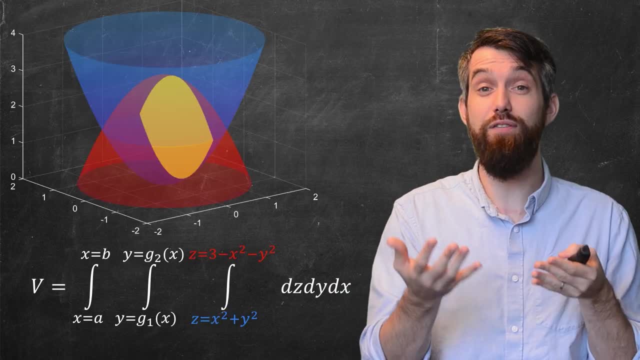 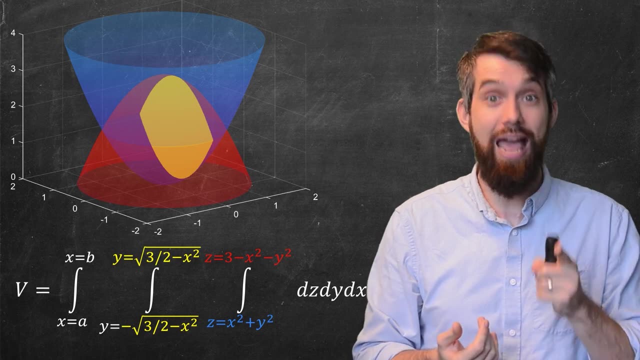 return, and what this is going to give me is it's going to give me this: g1 up to g2 is nothing but the square root of three-halves minus x squared with a negative, up to the square root of three-halves minus x squared with a positive. And then 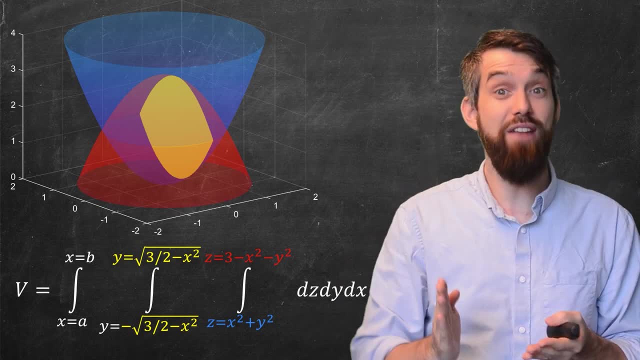 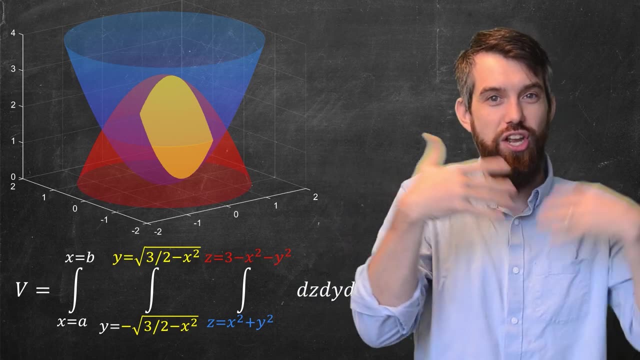 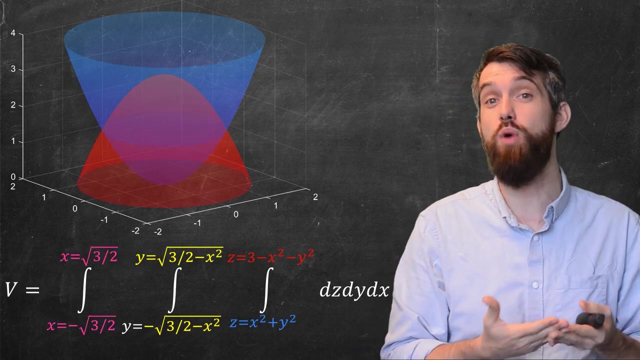 I take this combined slice so the z values changing and the y values changing give me this sort of weird two-dimensional looking thing. I imagine I change that as I change my x values. My x values are also going from the extreme ends of the circle, So they're just going between the minus square root of three-halves. 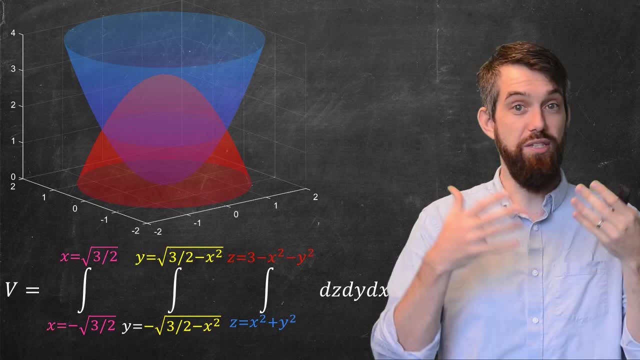 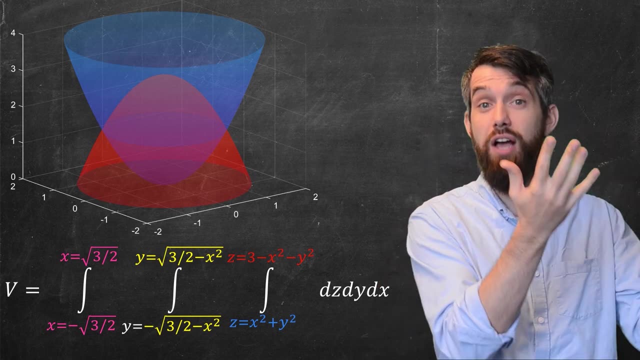 up to the plus square root of three-halves. This is now an interval and we've done the hard conceptual part of figuring out what the limits of integration are, And after this it's just a procedural process of evaluating it, which I will. 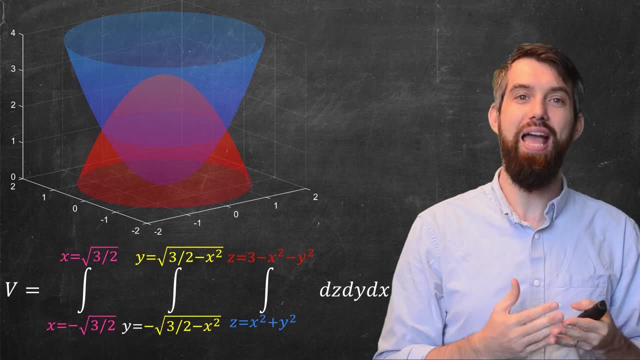 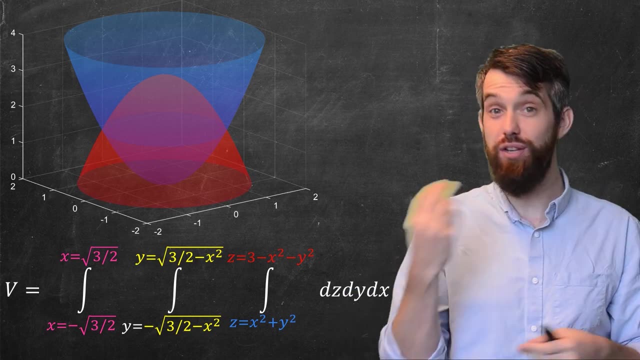 give to you. One observation about this is that as I integrate for z, this is a, then y, then x. The z limits of integration are functions of x and y, and when I integrate I get rid of any z, it's only x's and y's, Then the middle integral. 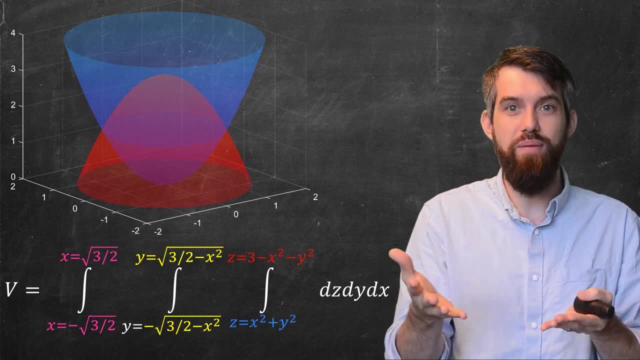 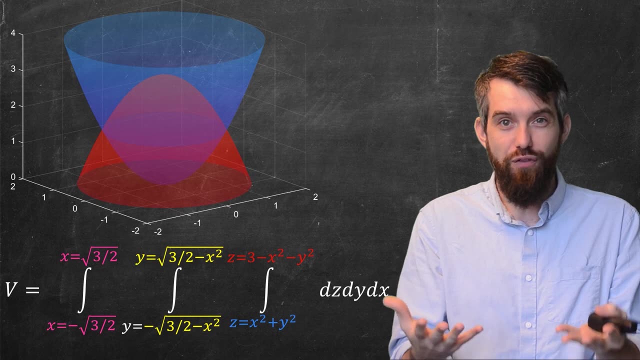 the one with respect to y. now the z is gone, but the y's can be written in terms of x's still. so my limits of integration are functions of x. I integrate with respect to y and I get rid of all y's. now it's just x's, And then the final integral, the one with respect to x, has.